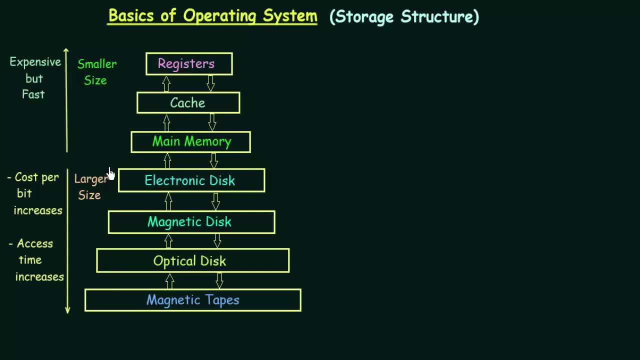 And if you go up to this, the size of the devices becomes smaller and smaller, But then their access time and cost it becomes higher and higher as we go up the hierarchy. So we can say that registers are the smallest in size but their access time is the fastest. 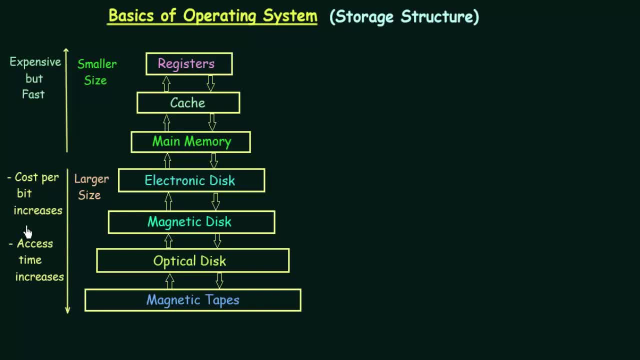 And as you go down the hierarchy, the cost per bit increases, The cost per bit increases And then the access time also increases And their size also increases. So we can see that if you want small size and fast access, then this is where you have to go. 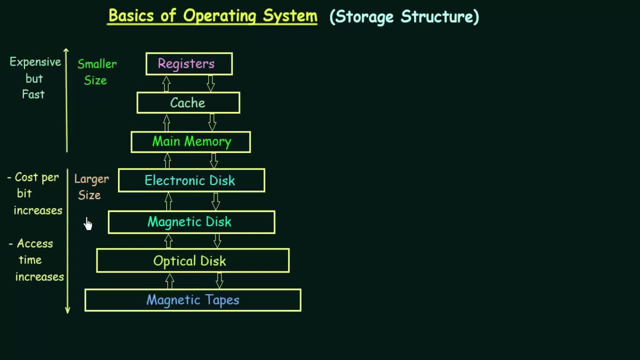 And if you want bigger size for storing more data, then you have to go down this hierarchy, coming to this electronic disk, magnetic disk, optical disk and magnetic tapes, And here the cost and the access time increases. Now, as we talk about this, we have to talk about our main memory. 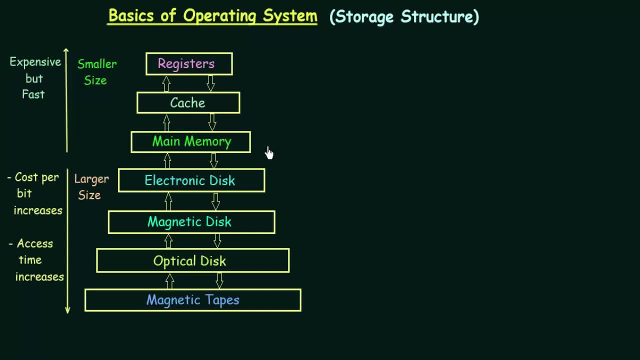 This is the most important thing that we need to talk about. So main memory is your RAM or the random access memory, And what is the function of main memory? In the main memory, anything that you load in your computer gets loaded to your main memory. 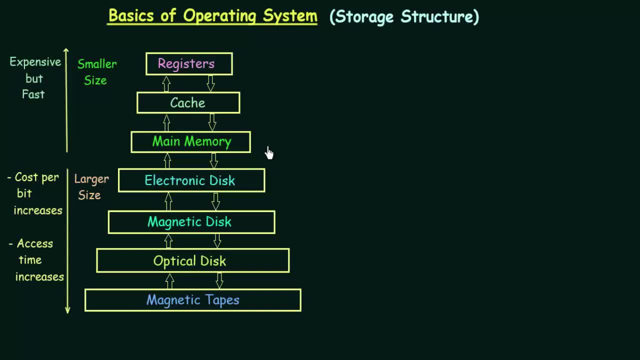 And that is where it is executed. So things are stored in your secondary memory, but things are loaded to your main memory for the execution purpose. Now, what do we mean by secondary memory? This main memory? it is fast, but its size is limited. 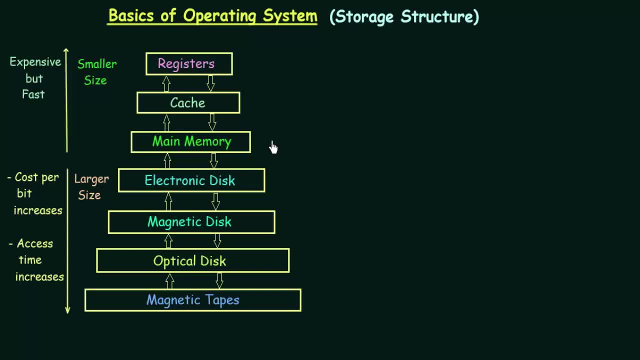 And also it is volatile in nature, And I will explain you what is the meaning of volatile. But remember that the size of this main memory is small, So you cannot store all your programs and data into the main memory. So for that purpose, 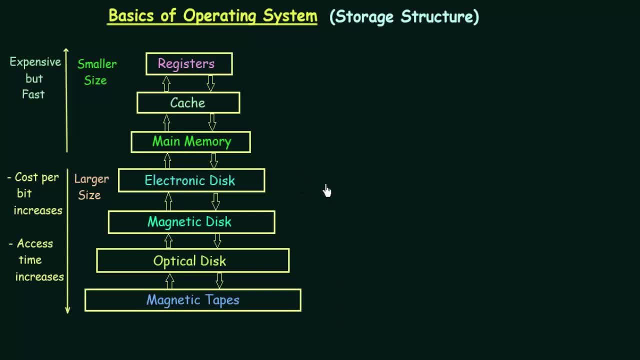 we have our secondary memory. So in our secondary memory we can store all our data and all other things that we need, And when it has to be loaded or executed, it is loaded into the main memory and then executed. So, for example, let's say that you have your word processing software. 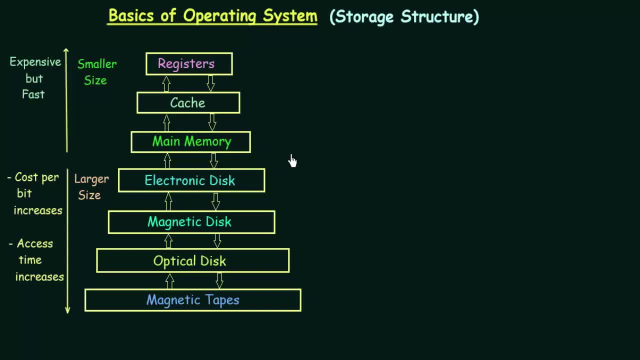 That is your Microsoft Word. So if you have your Microsoft Word it is installed in your secondary memory. It stays or resides in your secondary memory, But when you double click and open it, then it gets loaded to the main memory because you are going to perform some task in that Microsoft Word. 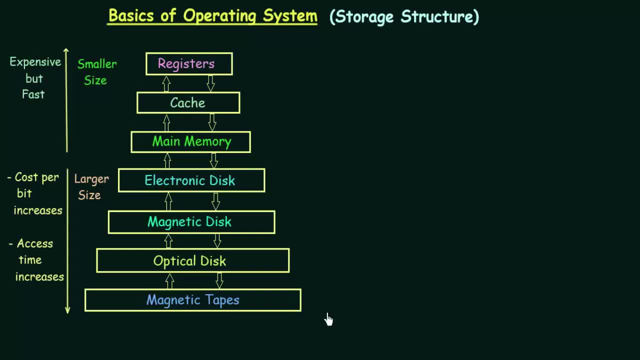 So whenever you execute something, it gets loaded in the main memory. Otherwise it is residing in the secondary memory. So all your data it resides in the secondary memory and it is loaded to the main memory at the time of execution. 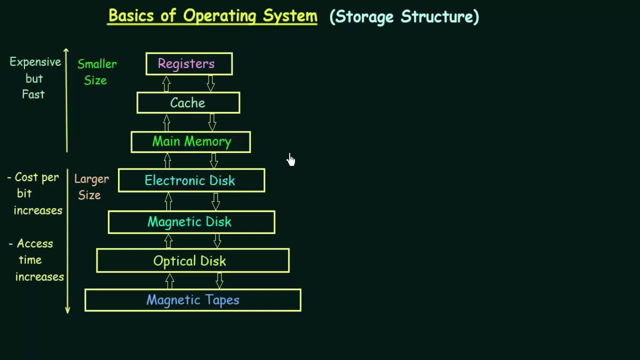 Now we say that when you have a larger or a bigger RAM, then your computer works faster. You must have heard this many times Now. why is that? Why do you say that when you have more of random access memory or RAM? 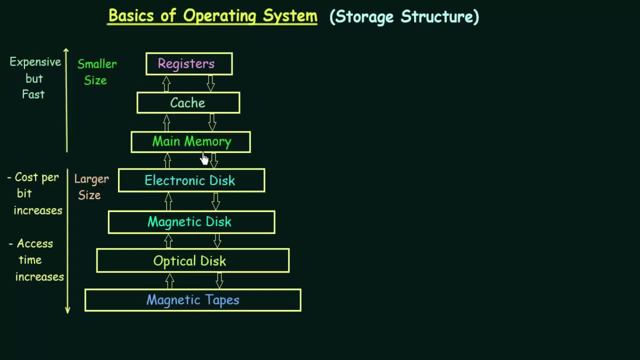 your computer is faster. So remember that main memory is your RAM. Your RAM is the main memory. So for explaining this, let me take a simple example. Imagine that you are in a room, in your study room, and then you have a bookshelf. 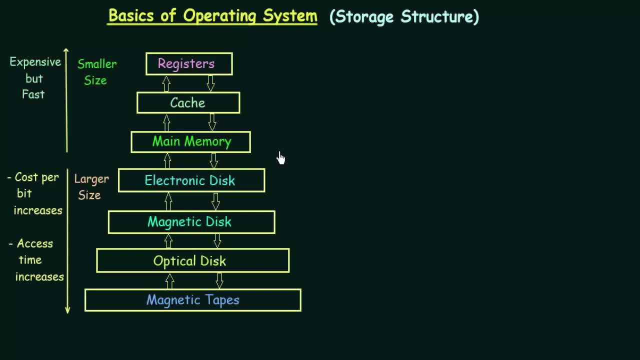 You have a big bookshelf where you can store many books, And then on that bookshelf you are having lots of books, And then beside you there is a table. There is a small table on which you keep your books for reading. 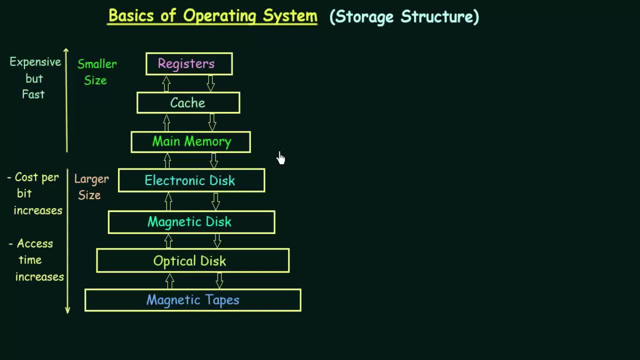 Now think of the bookshelf as your secondary memory and the books as your data. So all the data, that is, your books, are kept on the bookshelf. But when you want to read a book, what do you do? You take out the book from the bookshelf. 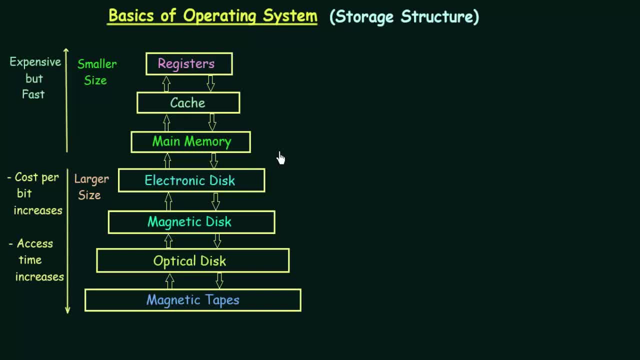 and you keep it on the table and then you read it. So just assume that you only read your book on the table. You don't like to read it in other ways. So whenever you want to read, you take a book from the bookshelf. 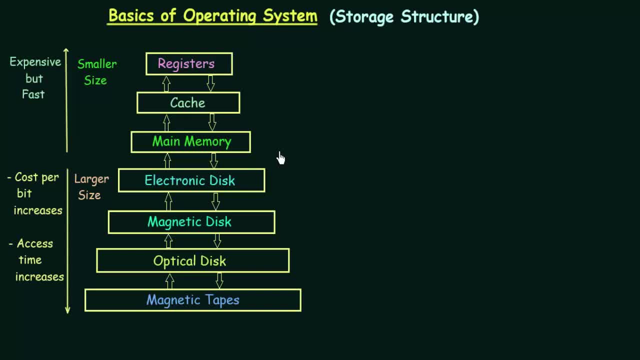 and you keep it on the table and then you read it And consider that table to be your main memory or your RAM. Now let's say that your table is very small. So if your table is very small, what happens? Let's say that you can keep only one book at a time. 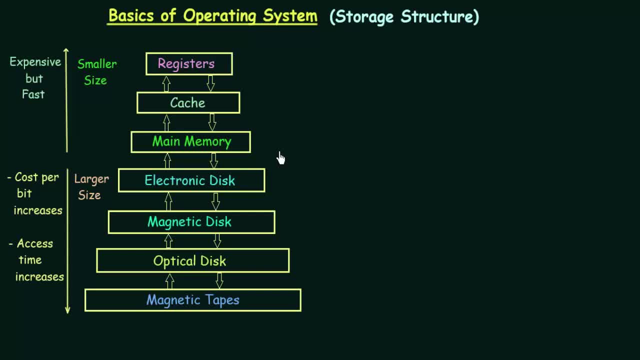 So if you can keep only one book at a time, you cannot use more than one book for studying. Even if you want to refer 2-3 books for studying, you cannot do because you can only accommodate one book on your table. 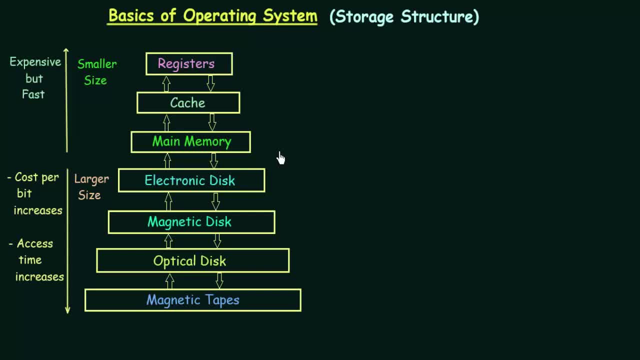 No matter how big your shelf is, the number of books that you can study at a time depends upon the size of your table. So the table- you consider it as your main memory. So in the same way, if you have a large secondary memory, 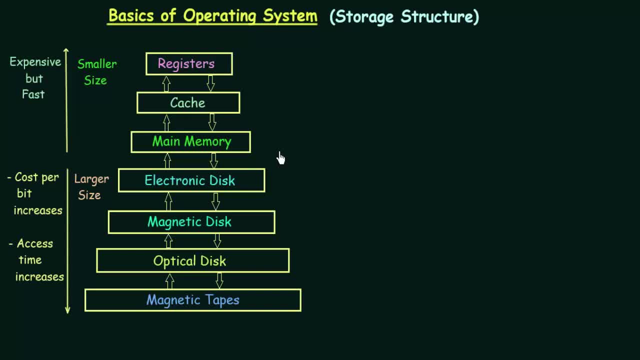 when you load things it is loaded into your main memory. So if you have a bigger main memory then you can load multiple things and your computer will work faster, And if you have a smaller main memory then the things will be loaded in a slower way. 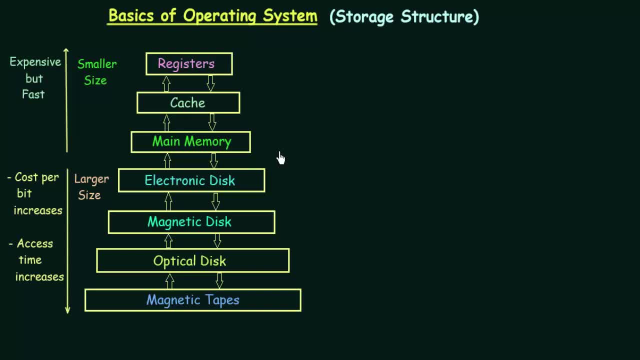 and your computer will be slower. So that is why you usually hear that when you have more RAM, your computer audio system performs faster. Now, as I was explaining to you, I said that main memory is volatile as compared to secondary memory. 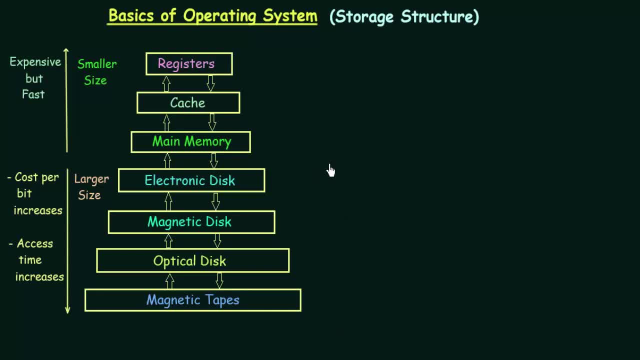 which is non-volatile. Now let us try to understand the meaning of volatile and non-volatile. So volatile means that it loses its contents when the power is removed. So all these devices, like your main memory cache and your registers. 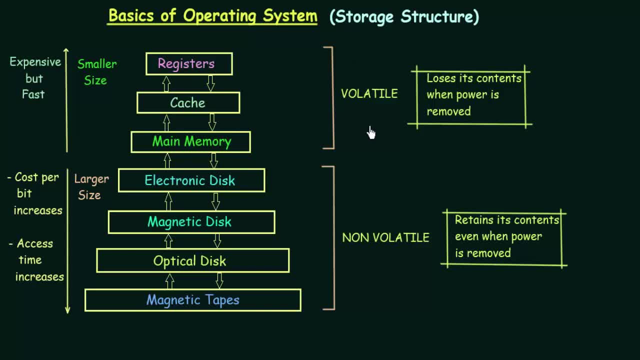 they are volatile in nature, which means that when the power to these devices are switched off, then whatever was stored in these devices will be removed or erased Alright, And, on the other hand, the secondary memory that you have. they are non-volatile. 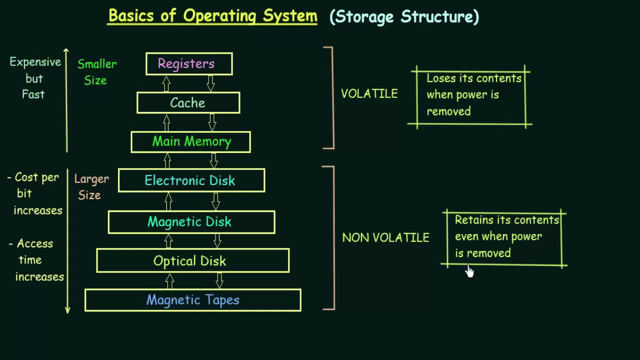 which means that it retains its contents even when the power is removed. So even if you switch off the power to these non-volatile devices, their contents will not get erased. They will be retained even when the power supply is removed. So here registers, cache and main memory. 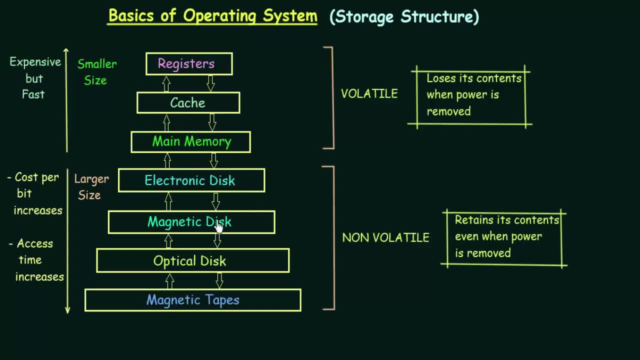 they are volatile, Whereas electronic disks, magnetic disks, optical disks and magnetic tapes, which basically are your secondary storage devices, they are non-volatile. This electronic disk, sometimes it can be made to be volatile as well as non-volatile.